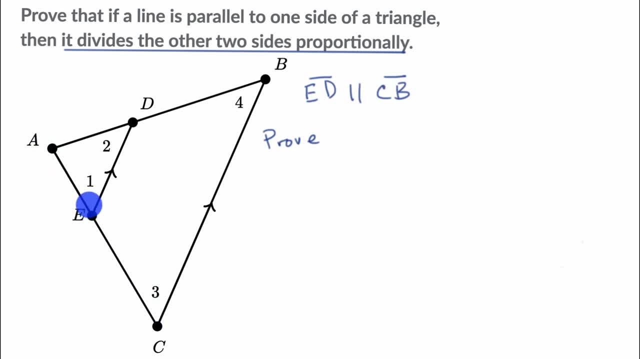 is that the ratio between the part of the original segment of the triangle and the original triangle side, that is, on one side of the dividing line to the length on the other side, is going to be the same on both sides that it is intersecting. So another way to say: 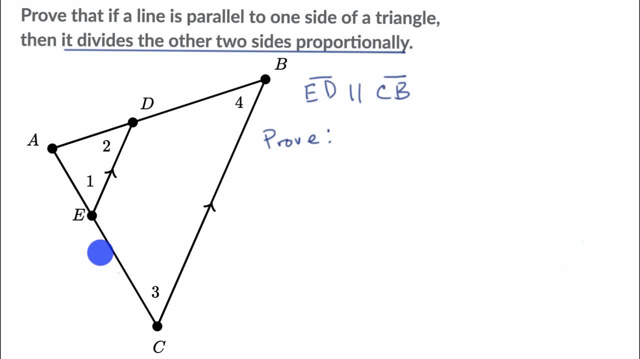 that it divides the other two sides proportionately. if we look at this triangle over here, it would mean that the length of segment AE over the length of segment EC is going to be equal to the length of segment AD over the length of segment DD. 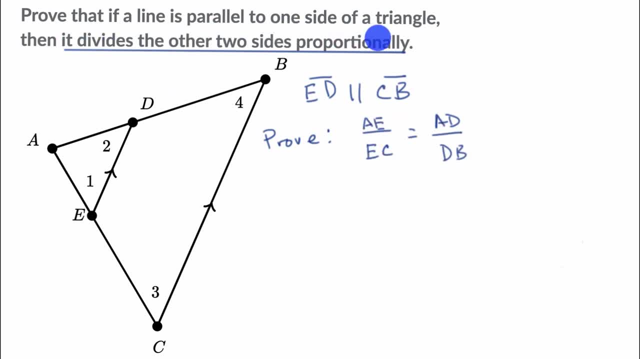 So the length of segment AD is going to be equal to the length of segment CB. This statement right over here and what I underlined up here are equivalent, given this triangle. So the way that we can try to do it is to establish a similarity between triangle AED. 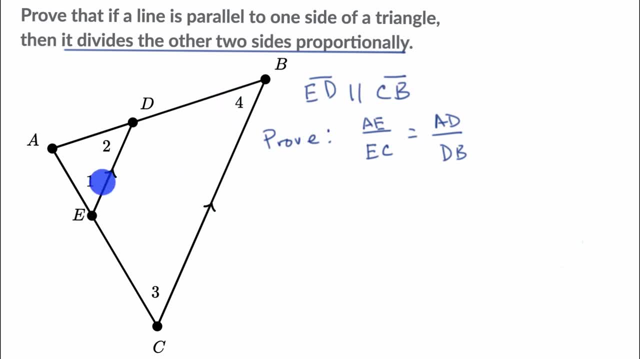 and triangle ACB. So how do we do that? Well, because these two lines are parallel. we can view segment AC as a transversal intersecting two parallel lines. So we can see that the transversal intersecting angles are going to be congruent. 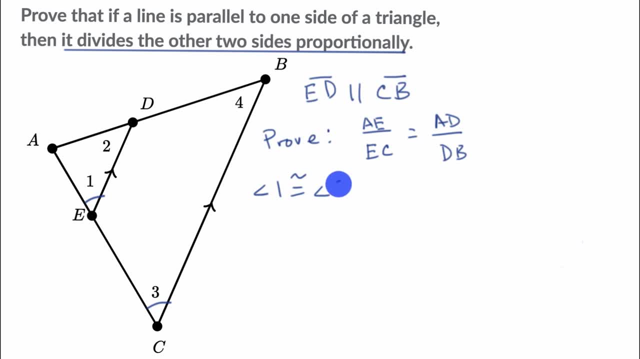 So we could say that angle one is congruent to angle three, And the reason why is because they are corresponding angles. I'm just trying to write a little bit of shorthand. This is short for corresponding angles. That's the rationale. And we also know that angle two is congruent to angle four. 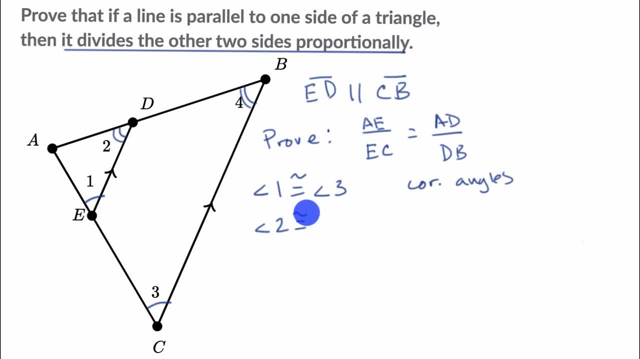 for the same reason, Angle two is congruent to angle four, once again, because they are corresponding angles. This time we have a different transversal corresponding angles where a transversal intersects two parallel lines. And so now, if you look at triangle AED and triangle ACB, 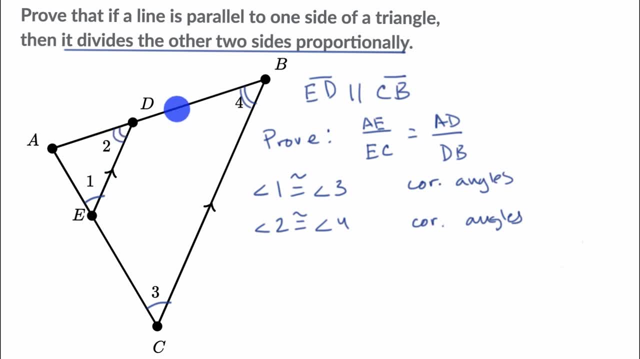 you see that they have two sets of corresponding angles that are congruent. And if you have two sets of corresponding angles, that means that all of the angles are congruent And you actually see that over here if you care about it. But two is enough, but you actually have a third. 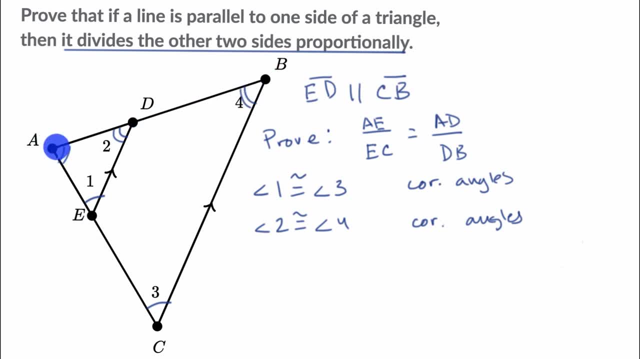 because angle- I guess you call it BAC- is common to both triangles, And so we can say that triangle AED is similar to triangle ACB by angle similarity. And then, given that these two are similar, then we can set up a proportion. 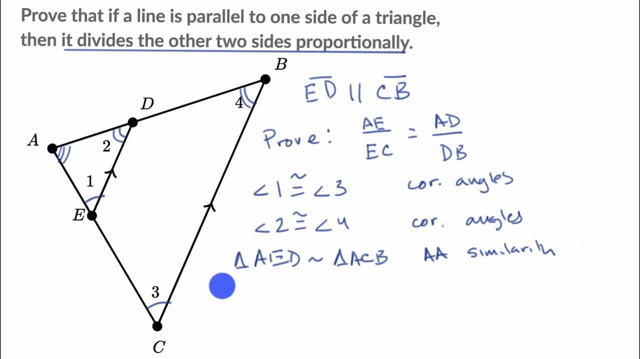 And that tells us that the ratio of the length of segment AE to this entire side to AC is equal to the ratio of AD- the length of that segment to the length of the entire thing- to AB. Now this implies- and I'm just gonna start writing it to the right here to save space- 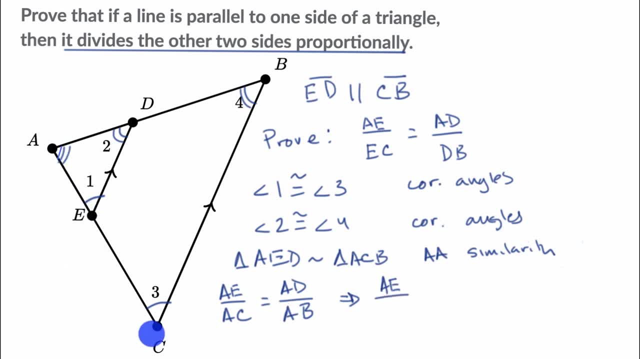 this is the same thing as the ratio of AE over AC is AE plus EC's length. So AE's length plus EC's length, And then this is going to be equal to the length of segment AD over segment AB. Its length is the length of segment AD. 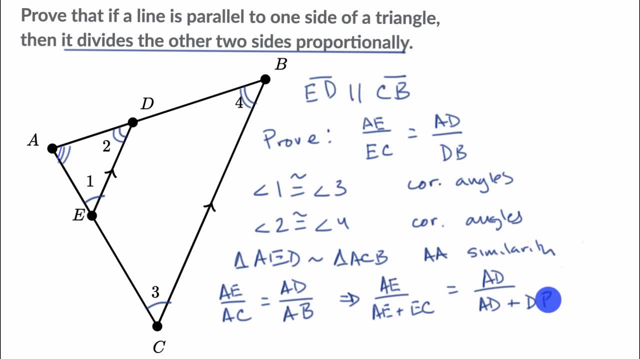 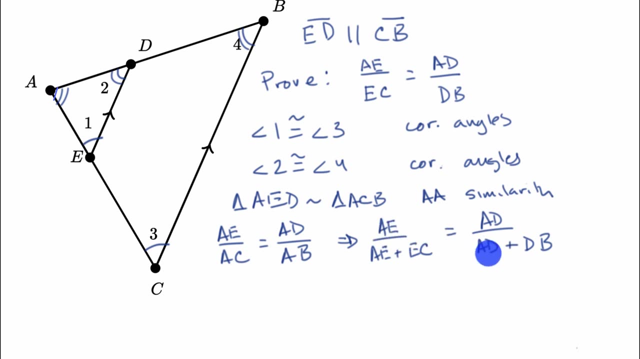 plus segment DB. Now, really, what I need to do is figure out how do I algebraically manipulate it so I get what I have up here. Let me scroll down a little bit. So one way I could try to simplify this is to essentially cross multiply. 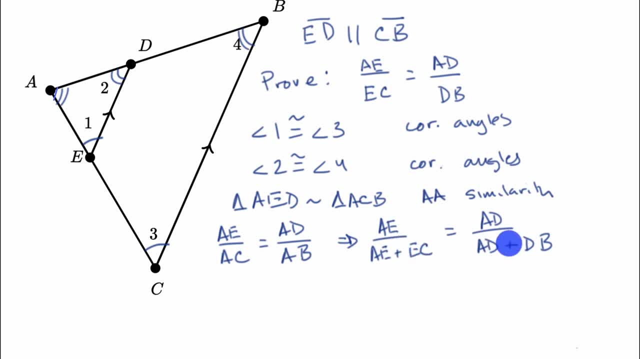 That's equivalent to multiplying both sides by both of these denominators, And we've covered that in other videos. And so this is going to be equal to the length of segment AE times, AD plus DB, those segment lengths. That's gotta be equal to. 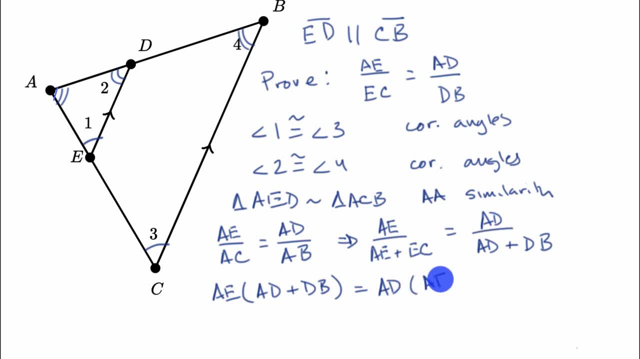 length of AD times AE plus the length of segment EC, And I can distribute this over here. I have length of segment AE times. length of segment AD plus length of segment AE times. length of segment DB is equal to length of segment AD times. length of segment AE. 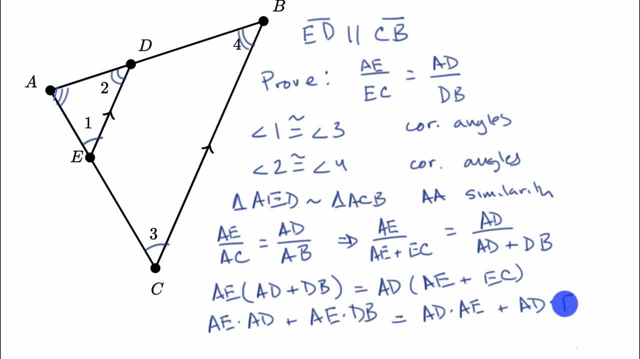 plus length of segment AD times, length of segment EC. And let's see, is there anything that I can simplify here? Well, I have an AE times AD on both sides, So let me just subtract AE times AD from both sides, And so then I'm just left with the. this is equal to that. 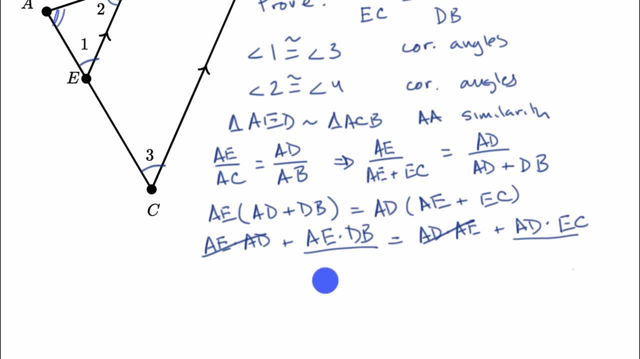 So scroll down a little bit more and let me actually just rewrite this cleanly. So I have AE times. DB is equal to AD times, EC. These are all the segment lengths right over here. Now if you divide both sides by EC, you're going to get an EC down here.